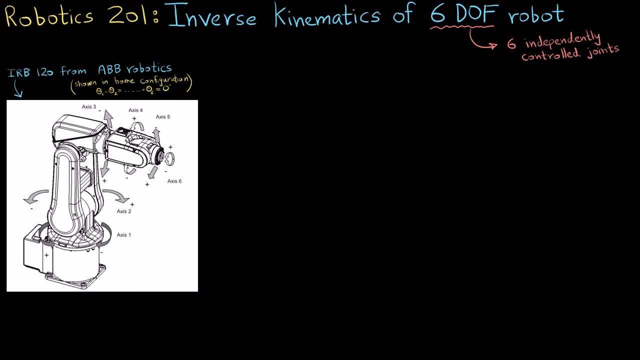 that we see it currently, it is in home configuration. so now, what is inverse kinematics? so in inverse kinematics, you are given the end effective position and orientation and you have to determine the joint parameters. in this case, what angles of the motors would you like? what? what commands would you need to give the motors in order to? 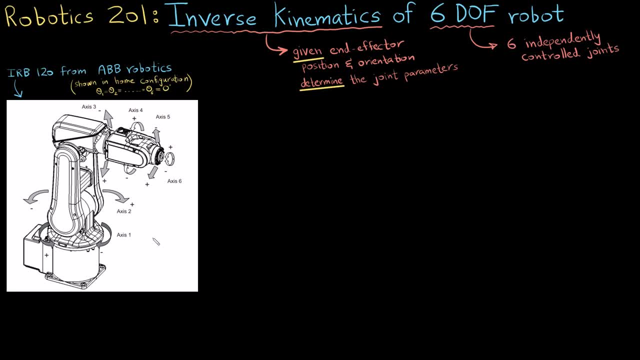 make the robot go to a certain position with a certain orientation. you can think of it this way, like if you have a pick and place operation in an industry and you have this robot right here and the object that it needs to pick is right here, so you will. 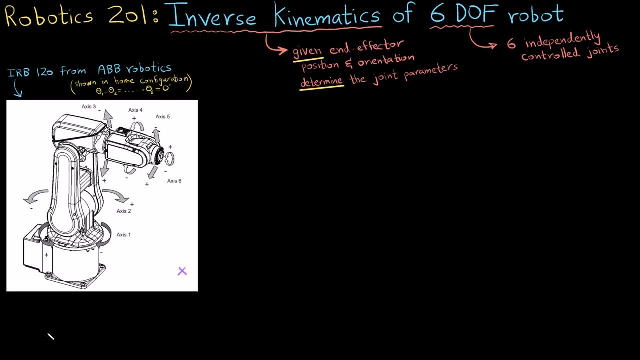 know the position of the object with respect to some reference frame, let's say with respect to this reference frame x, y and z. so we can say that this object is some units in x, some units in y, some units in z. so we know the position of the object and we know that you know. 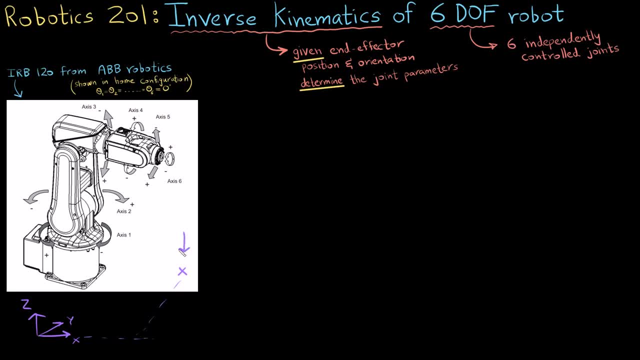 the origin of the object and we know the orientation of the object and we know the angle of the point of the object and therefore, in order to pick the object, the robot needs to approach it in this direction, from this orientation. so now we know the position and the orientation. 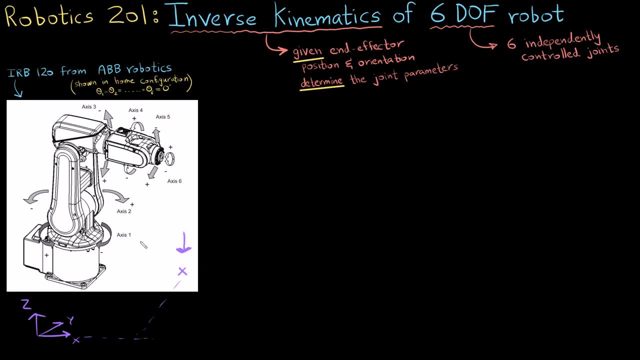 now we would need to move backwards and figure out what motor commands do we need to give to the motors, what angles should be the motors at in order to achieve this position, orientation and pick the object. so in the question that we have today, we are given homogeneous transform and we have to figure out the joint parameters. just to quickly recall what 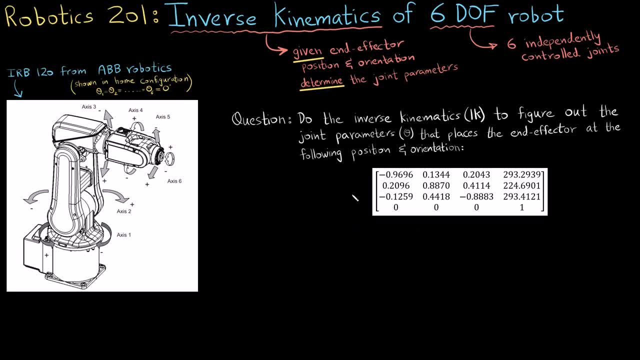 does a homogeneous transform represent? the homogeneous transformation basically represents two things. we can state it shortly in this form: so the bottom row is always three zeros and a one and the first three cross three matrix is the orientation matrix. which is this the orientation, and this the last three cross. one vector is the. 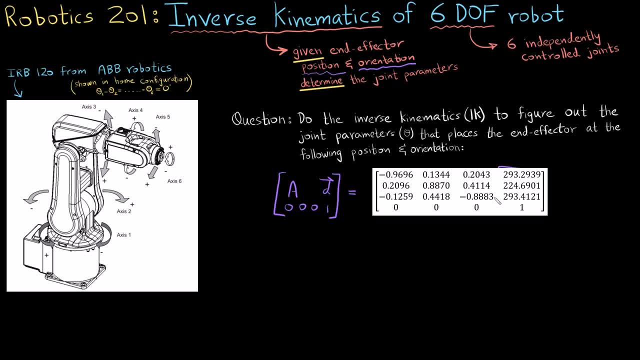 displacement vector or the position vector. so right here this one. right here is the- sorry, not this one, but this one. right here is the position. so this shows me the x, y and z coordinates of the location that the robot needs to be, the end effector of the robot, and this tells us the orientation. 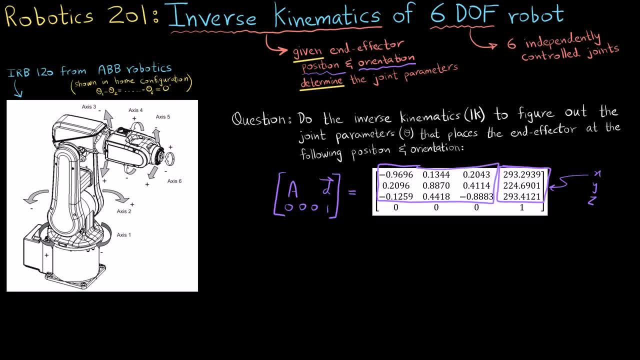 so how do we proceed with the inverse kinematics? but before we proceed with inverse kinematics, we need to understand. when someone has given us this inverse kinematics homogeneous transform, they have defined a reference frame, frame in which they have defined these x, y and z coordinates as 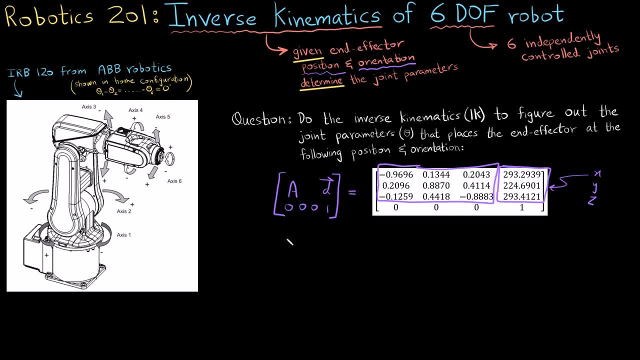 well as the orientation. so there are two reference frames of importance. the first is a base frame and the second is the end effector frame. so, right here, this one is my base frame, or i can. often it is also called world frame. they may or may not be the same, but for this 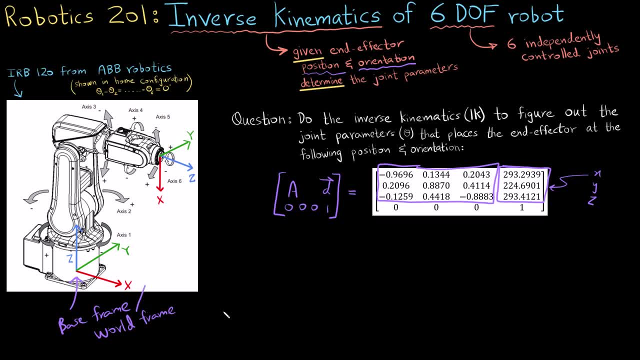 question. we are assuming them to be the same base frame or world frame. so what we are doing is the x y z coordinates are defined with respect to the base frame, the world frame, so some units and x and z- and this is my end- effective frame. so i need this frame and effective frame to move to this x y z coordinate and at this orientation, 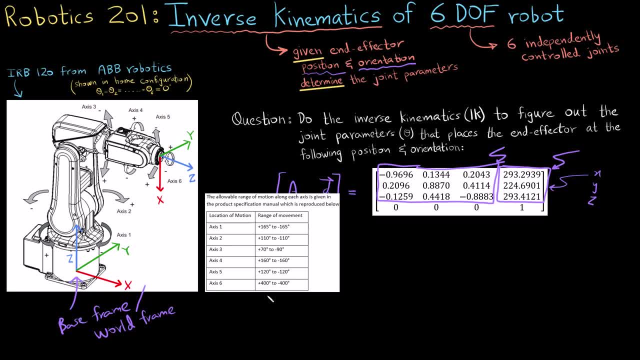 now, from the product specification manual, i have picked out this chart which just shows you how much the motors can rotate in every direction. and since it is a physical robot, it makes sense that the motors cannot rotate equally in all directions. this is due to physical constraint. so how do we go about inverse kinematics? there are four basic steps. 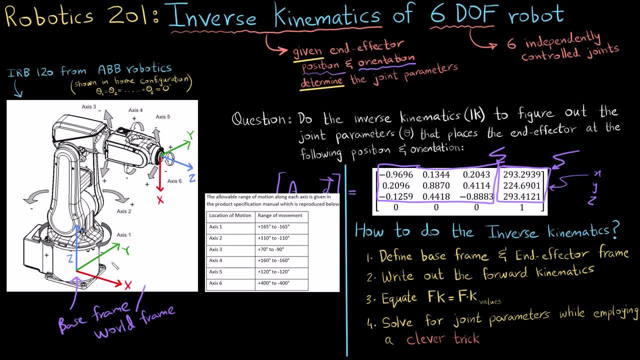 that we need to do, the first being we need to define the base frame and then effective frame, which, in this case, i have already defined: the base frame and then effective frame. secondly, we need to write out the forward kinematics. thirdly, we equate the forward kinematics. 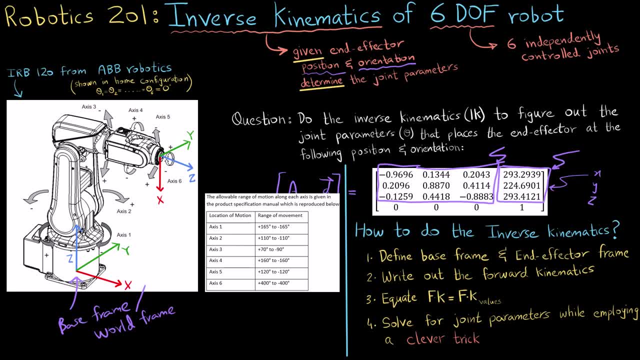 to the forward kinematics we use, which is this metric right here. so we write the forward kinematics沒錯, we escreve forward kinematics pudding to forward kinematics monitoring framework. we write forward kinematics, forward kinematics to the corresponding layer value and we do x, x, y, xель, x, el.